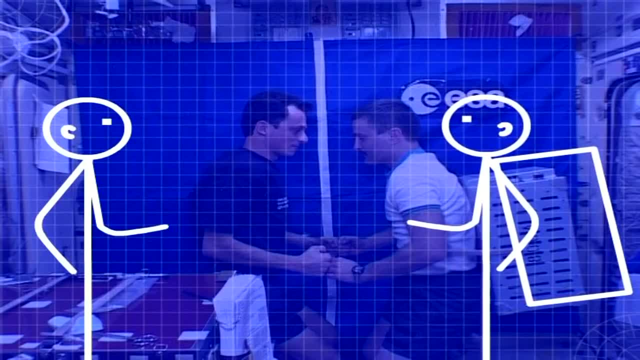 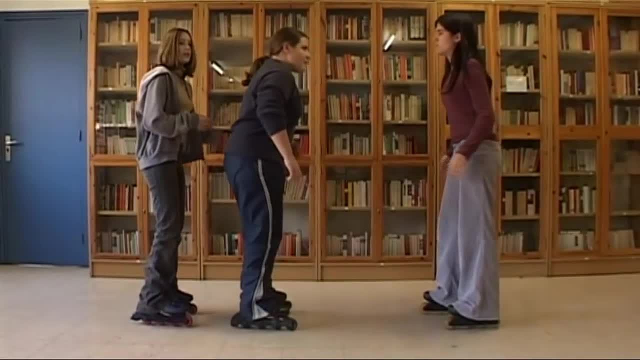 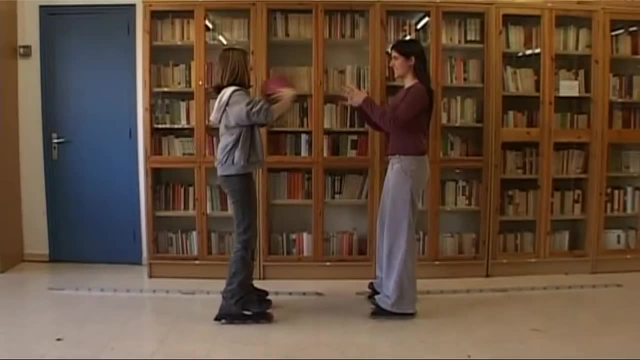 Therefore, Alexander moves less. Let's see what the schools are up to. Here we go. This is like Pedro and Alexander on board the station. We add another girl and they don't travel as far. The force of throwing the ball makes her move backwards. 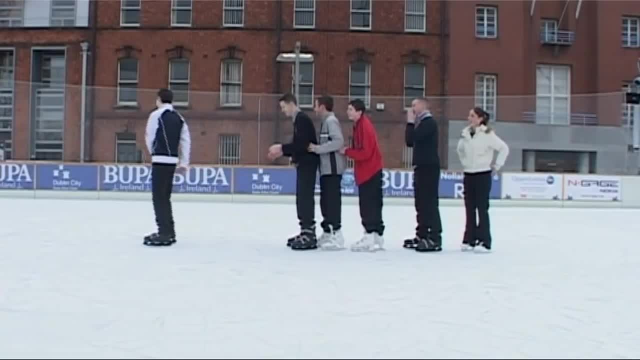 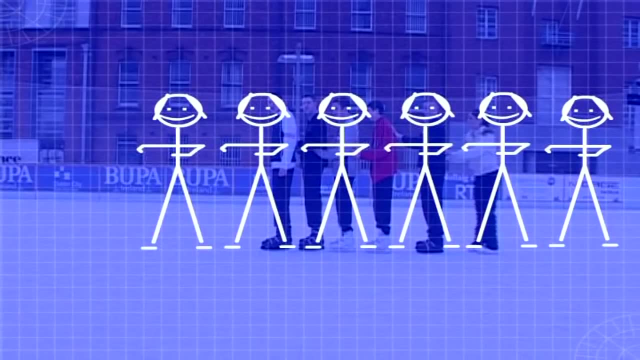 A collision. That's a force, But do you know why? Why only the guy in front moved. The students are arranged in what we call a Newton's cradle. Skater collides with the first student Action. The first student tries to move away from the skater. 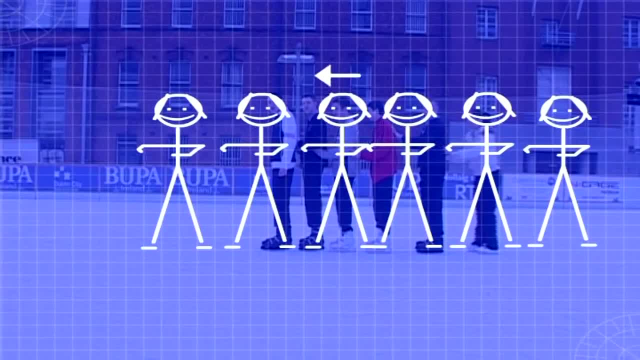 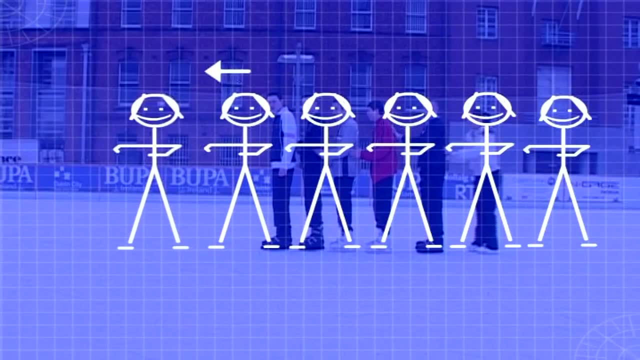 Reaction, But can't Because there is another student in the way. So the force of the impact is passed through the next student and onto the end of the line. Then there's nothing stopping the last student, So off he goes. 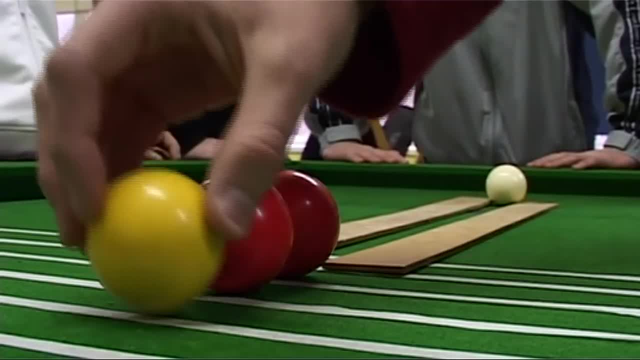 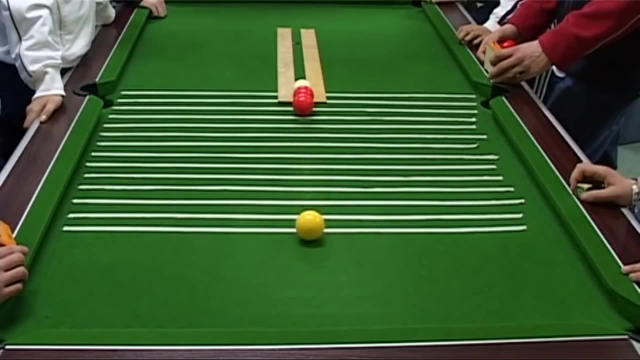 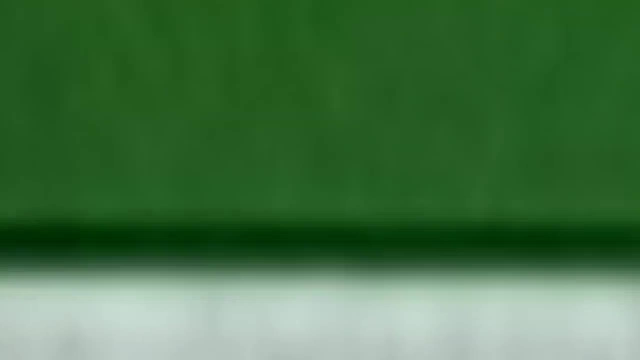 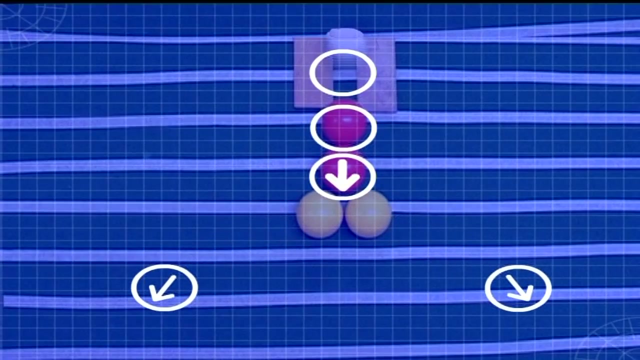 This is like the guys on the ice: Only the last ball moves. And here the two balls are moving, but they don't seem to go as fast. This is because the same force is travelling through the cradle, but is expressed through twice the mass. 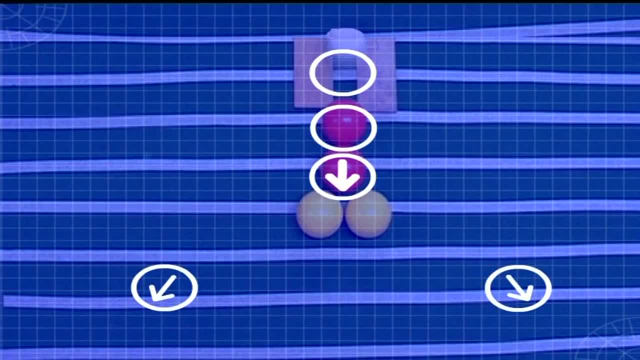 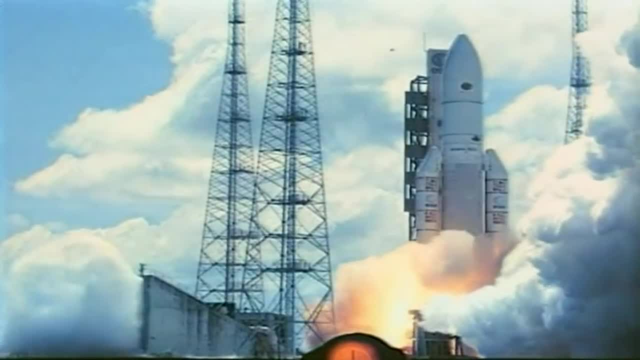 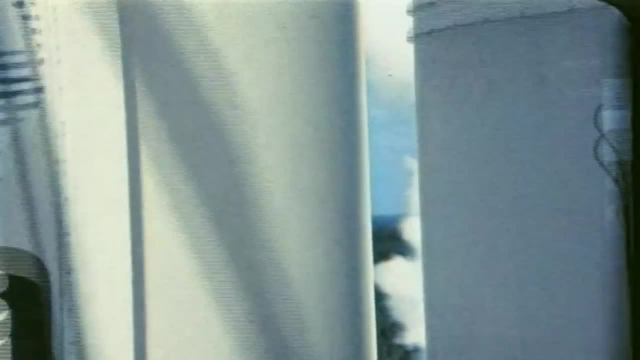 As mass and acceleration are related, the two balls travel less than the single ball. The third law helps us in other areas too. Space vehicles use it to lift off. The air or gas is heated up and forced from the exhaust Action, And the reaction pushes the rocket up into space. 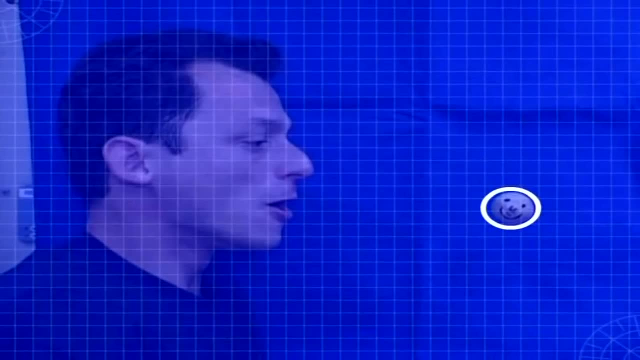 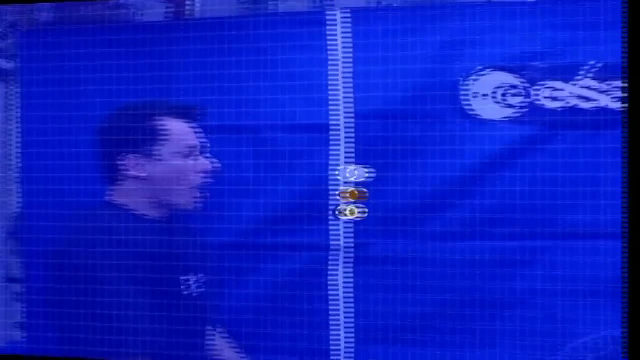 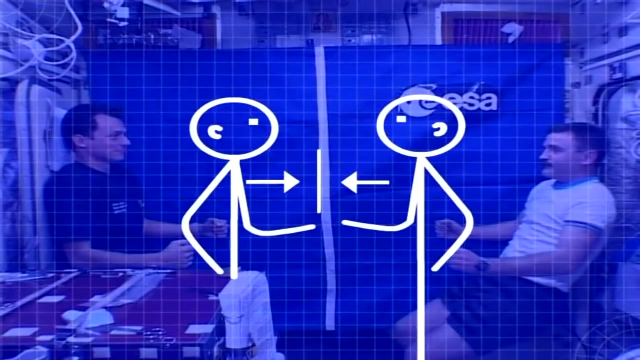 Now you know about Newton's three laws of motion. Law one states that objects at rest or in motion stay that way unless a force acts on them. Law two says that the force is related to mass and acceleration. And law three says that every action has an equal and opposite reaction. 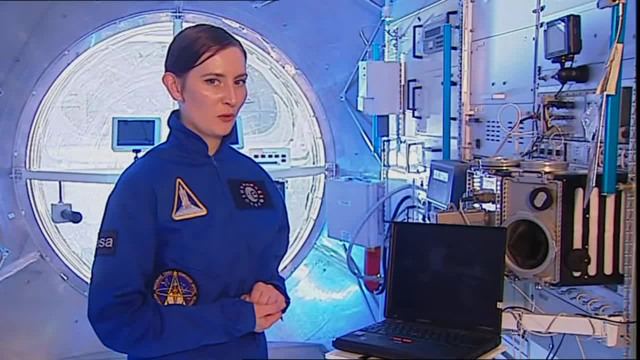 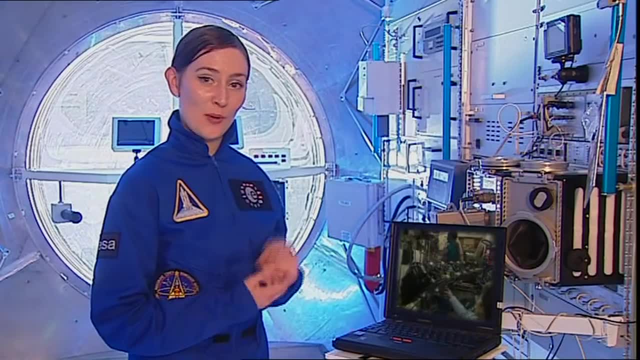 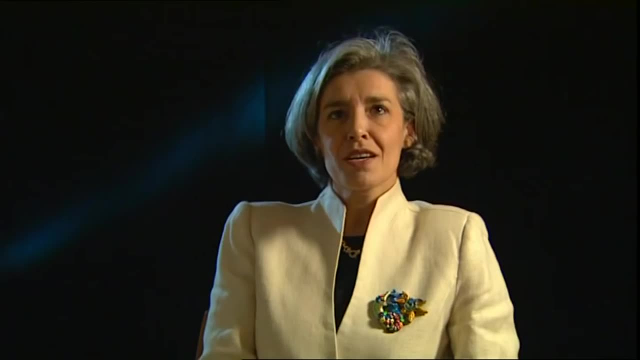 But why should we learn about Newton's three laws of motion? Well, it's all about science and research. Let's ask someone who has been into space. Hello, I'm Claudie Aignieret. I've been lucky enough to lead a fascinating life.